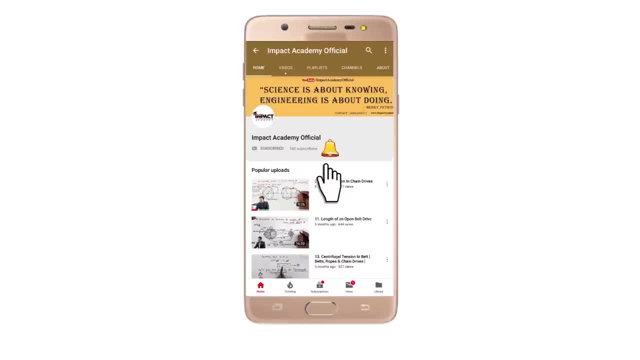 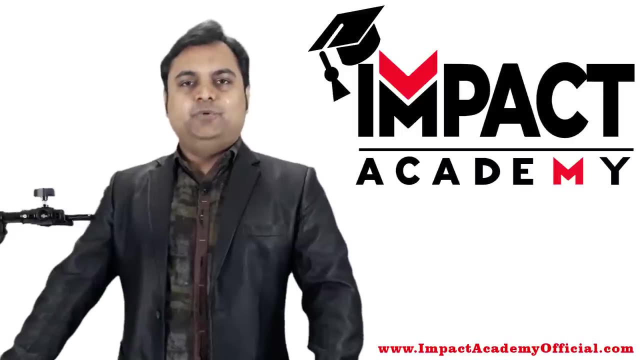 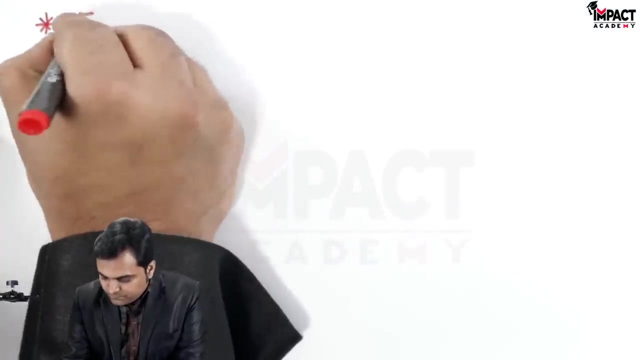 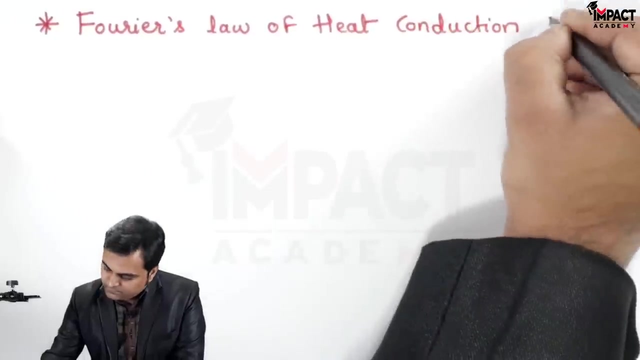 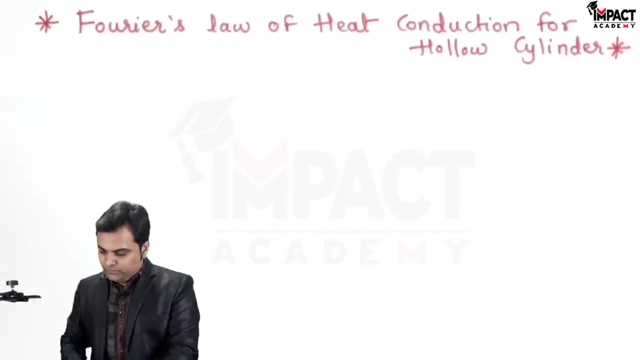 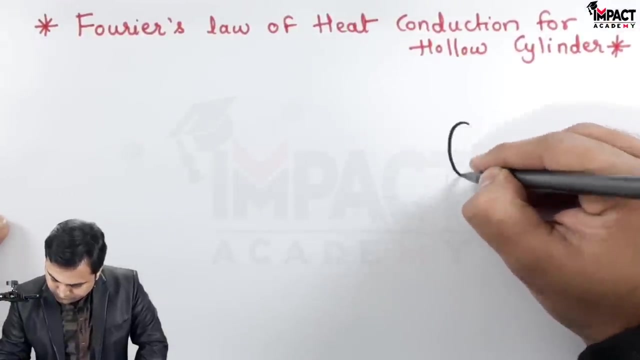 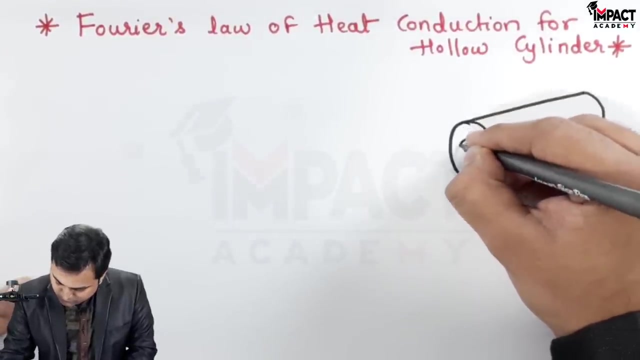 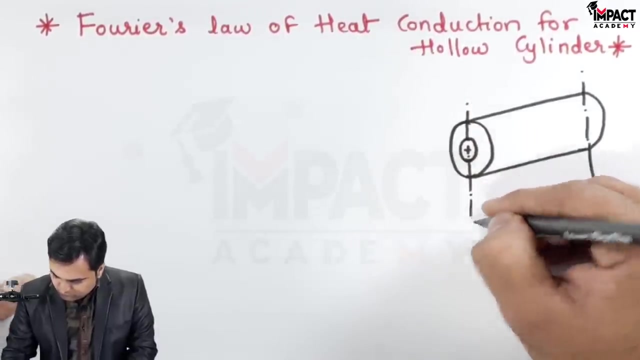 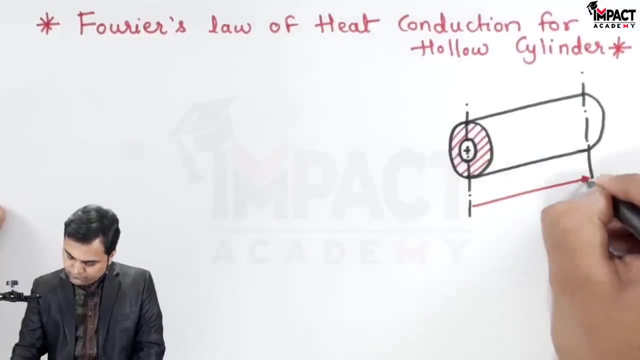 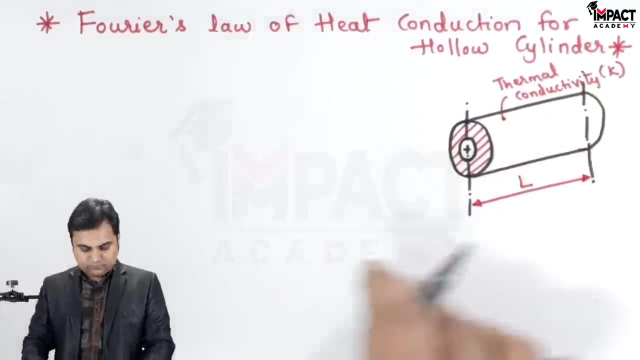 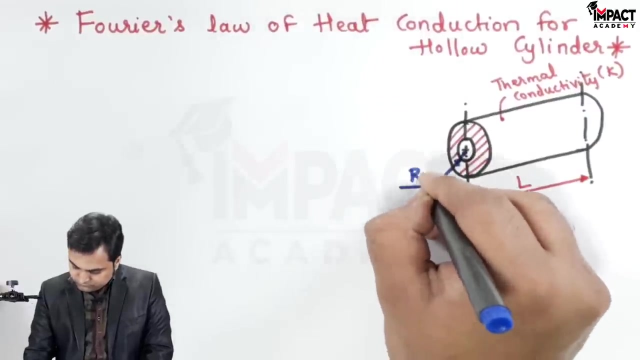 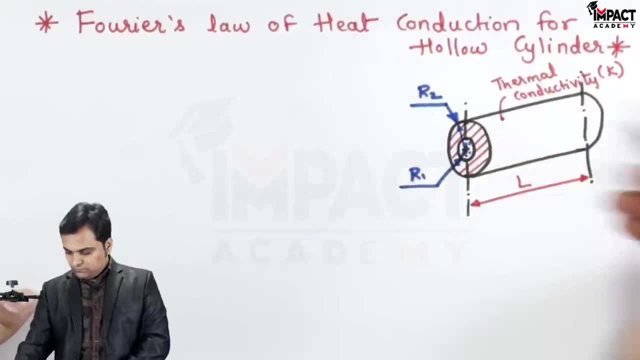 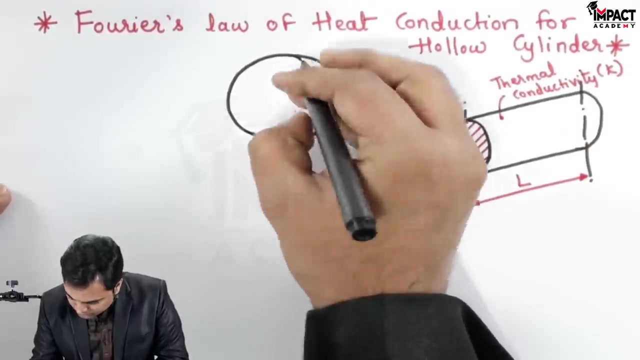 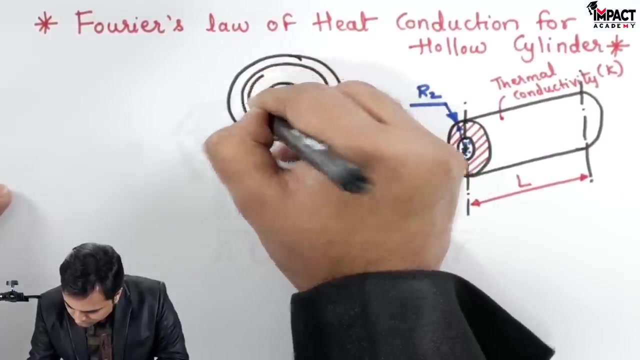 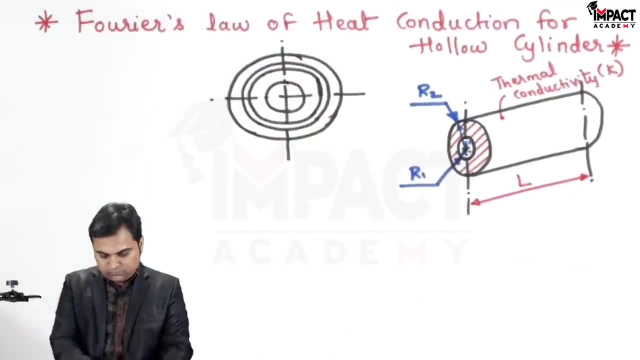 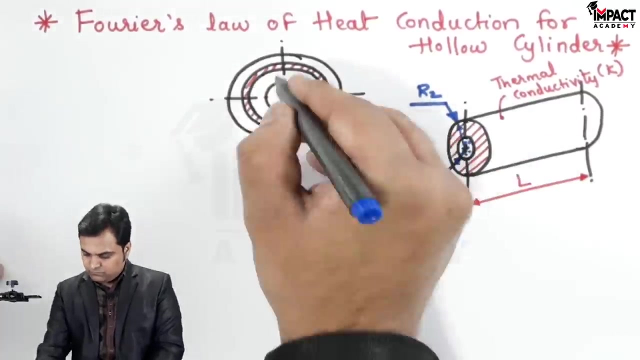 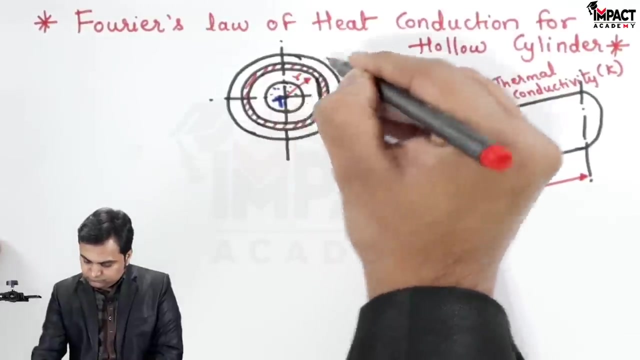 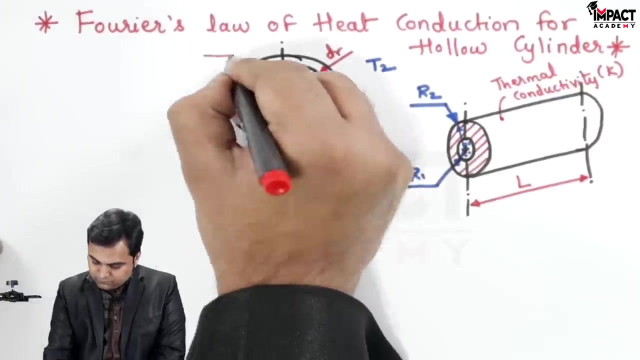 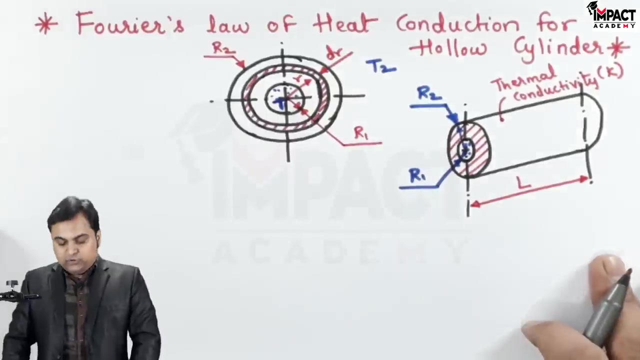 Subscribe our channel. Press the bell icon for latest videos. First, I'll quickly draw the diagram of the hollow cylinder. I'll draw the shape of the hollow cylinder you so? here there is a diagram of a hollow cylinder in which there is a fluid inside the cylinder. 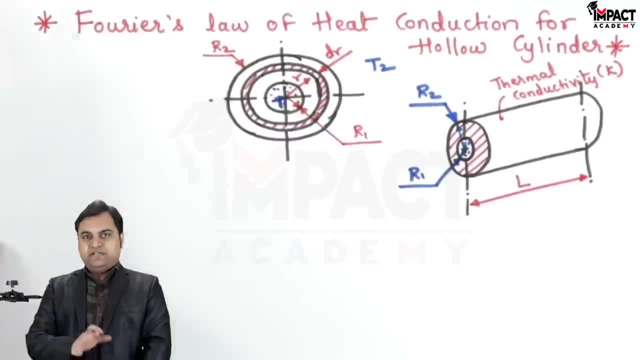 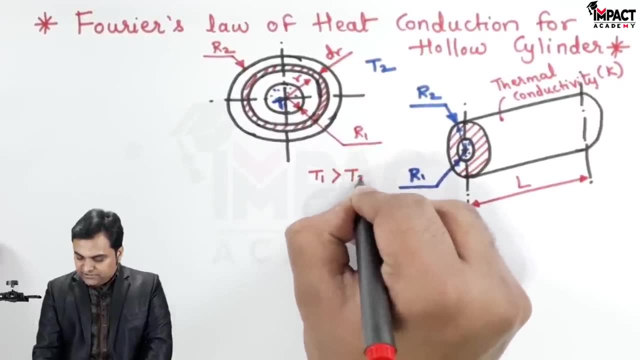 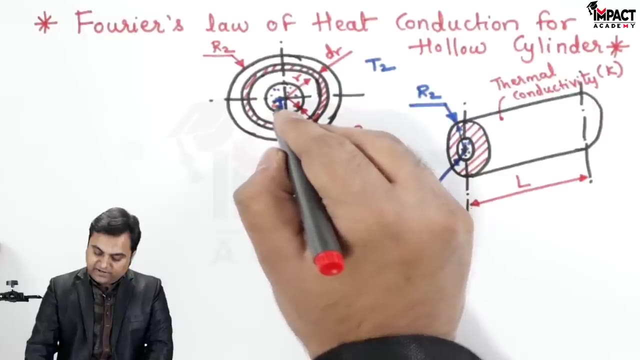 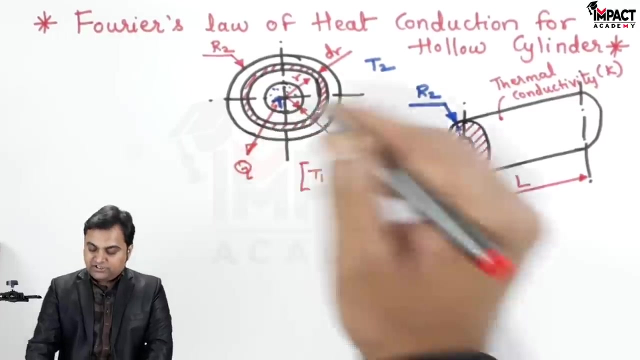 and having high temperature in the inside. that is the assumption which i am taking. inside temperature is t1 and the assumption is t1 is greater than t2. t2 is the outside temperature. so heat is getting transferred from inside to outside through conduction that is passing through this cylinder. wall cylinder is having internal radius. 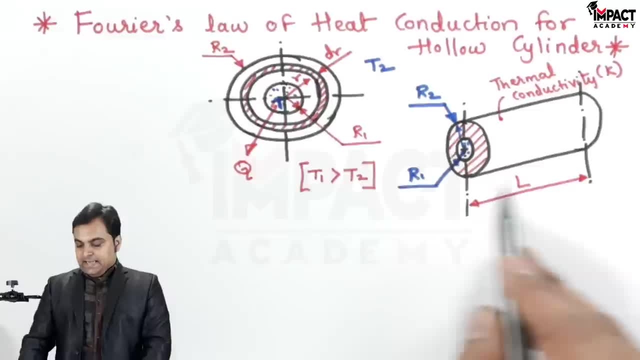 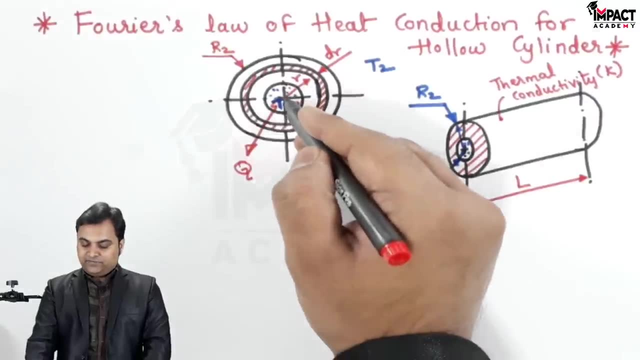 of r1 and external radius of r2. at the same time the cylinder is having length, capital l. its thermal conductivity is k. in this cylinder i am considering a ring at a small radius of r1 and external radius of r2 and external radius of r2 and external radius of r2. and 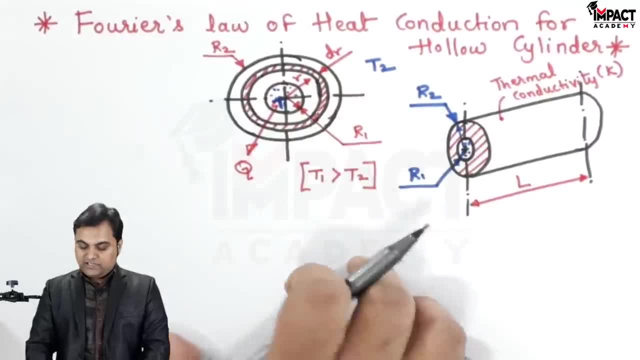 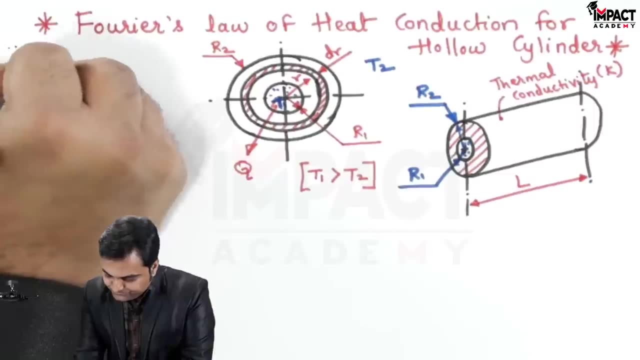 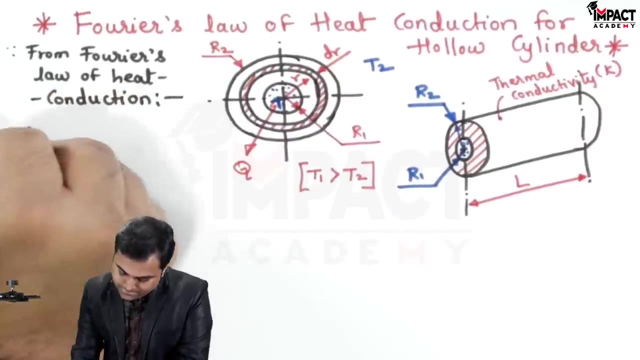 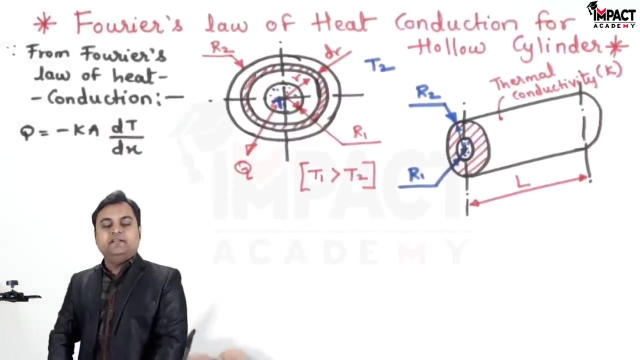 external radius is r, which is having thickness dr. so i will start the formula from the eğ Height conduction, since the desertedijn law of heat conduction is minus kad by dx, and how this comes from. for that you all can refer my video in which i had explained the 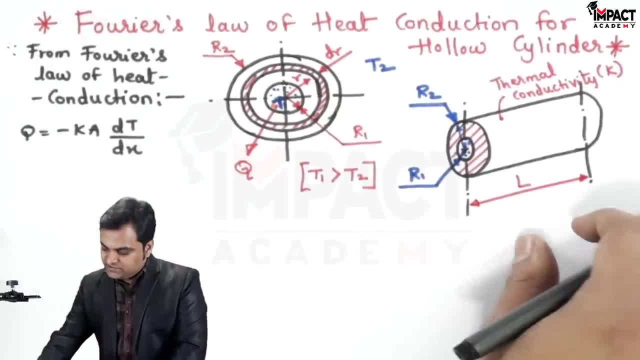 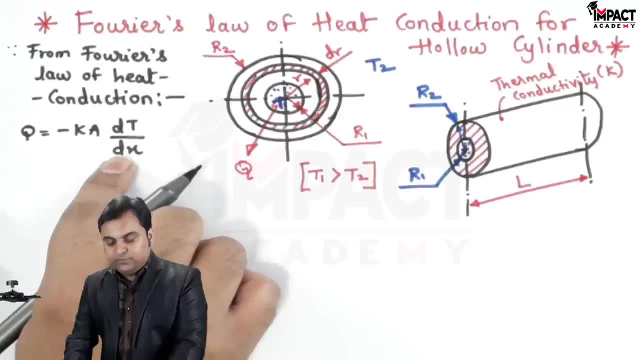 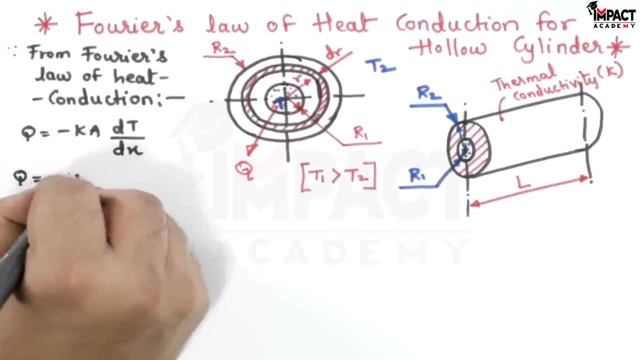 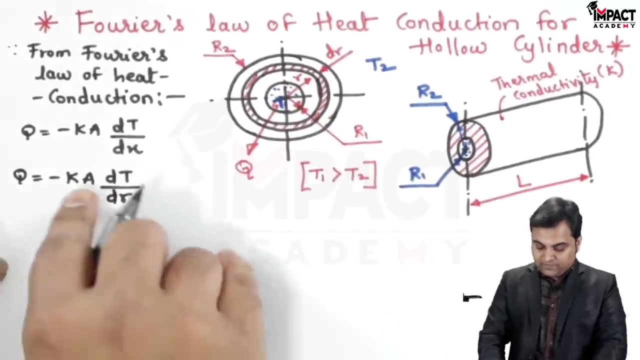 furious law of heat conduction. next, since this is a cylinder, and here the law is written, for a plane wall having thickness dx, this dx would be replaced by the radius, which is dr, so this equation would become minus ka dt by dr. for a hollow cylinder, then the area of this cylinder which. 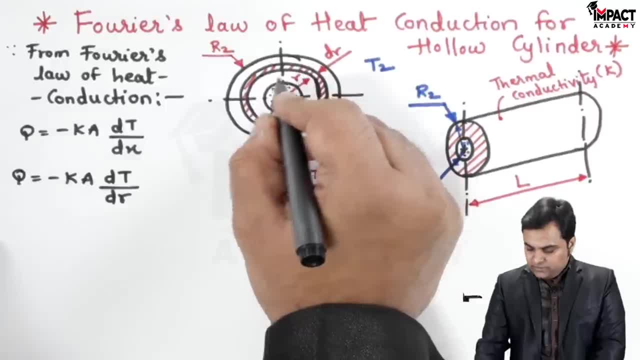 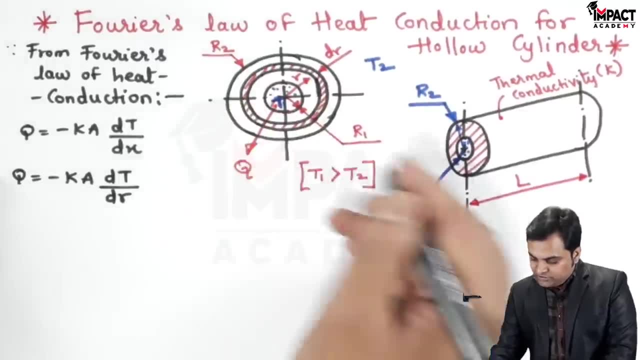 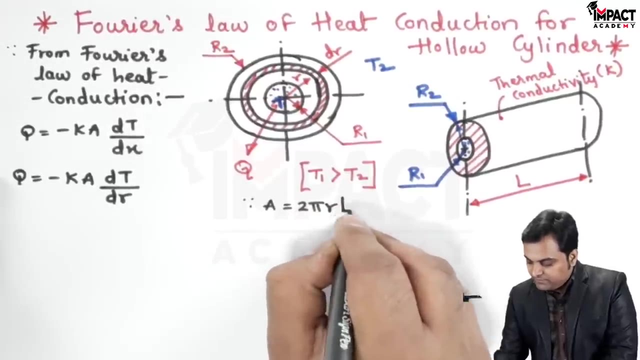 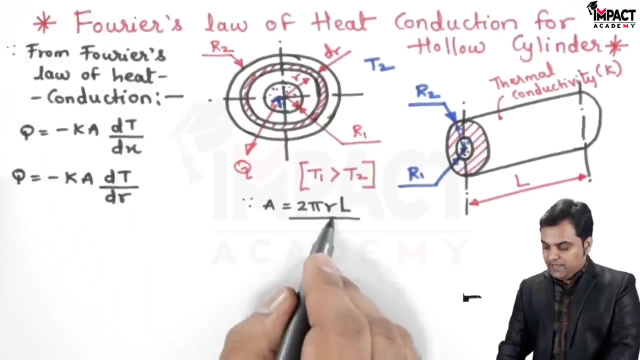 is located at radius small r, because i have to take the area of this small ring, then i'll equate it for the complete hollow cylinder. so here the surface area is 2 pi into small r multiplied by the length of the cylinder that is the area of conduction heat transfer, 2 pi r into l, so putting 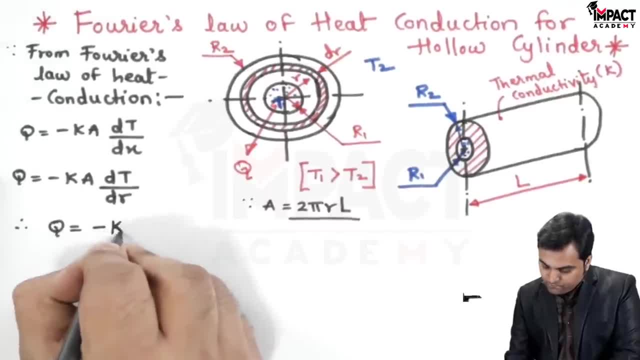 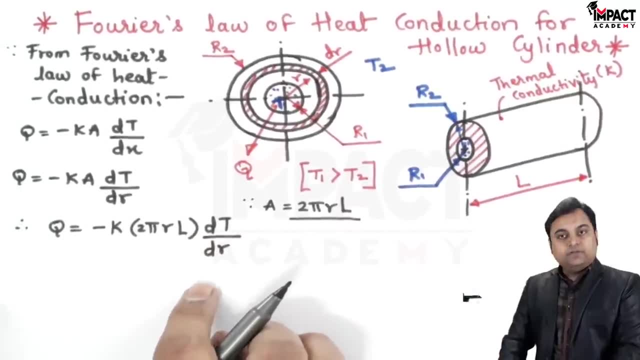 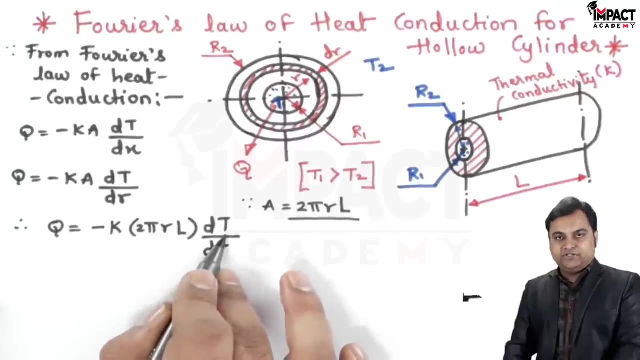 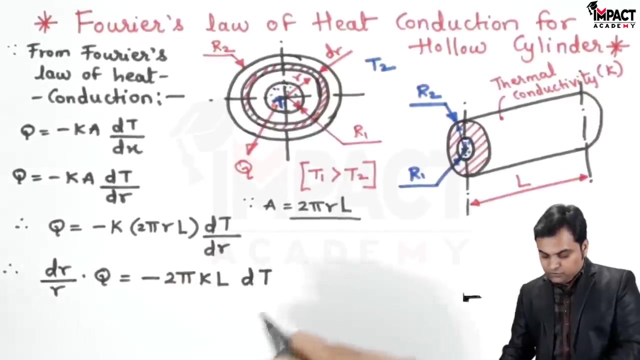 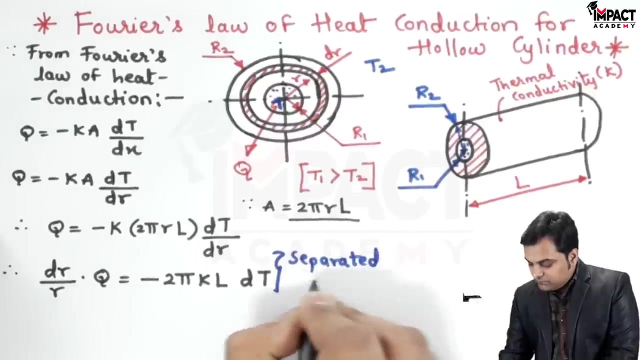 the value dt by dr. now i would be separating the variables, and in this equation the variables are radius and temperature. so therefore q would be kept over one side. dr would be multiplied here. so dr upon r into q is equal to minus 2 pi kl into dt. so here what i have done is i have separated the variables. 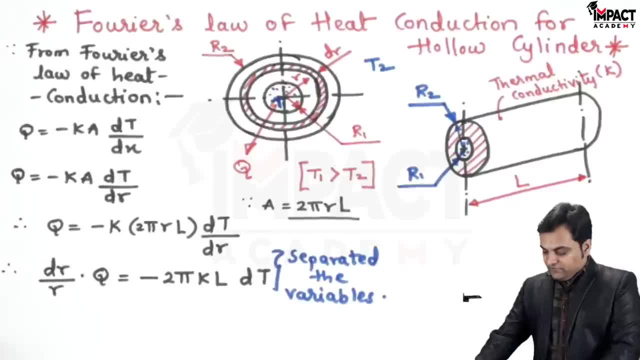 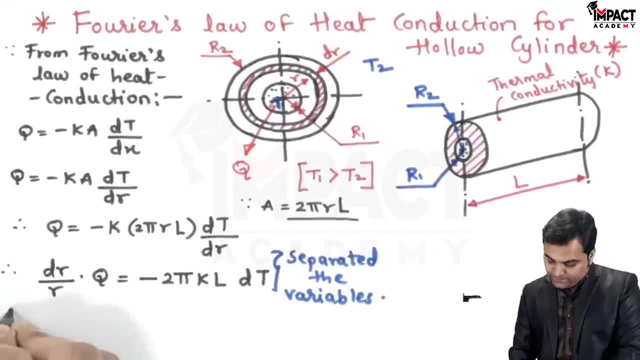 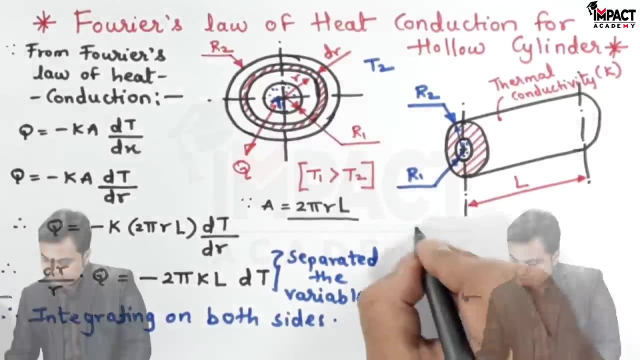 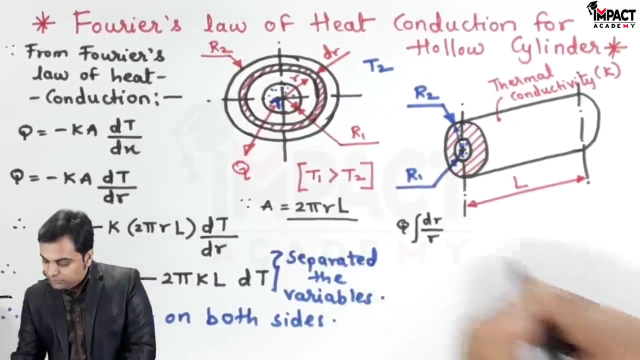 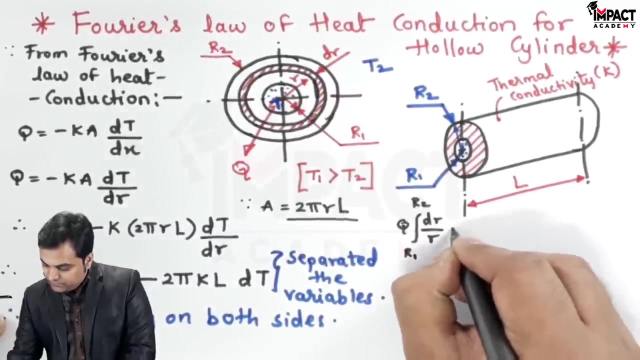 next, after reaching up till here, i would be integrating this equation on both sides to get the total rate of heat transfer. q will remain as it is. it would be: integration of dr upon r, and the limits are from r1 to r2 is equal to minus 2 pi kl. integration of dt. 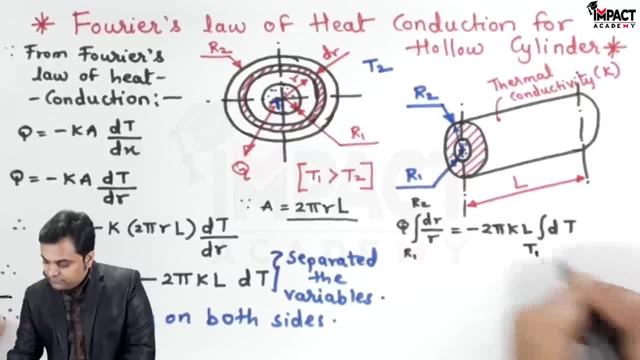 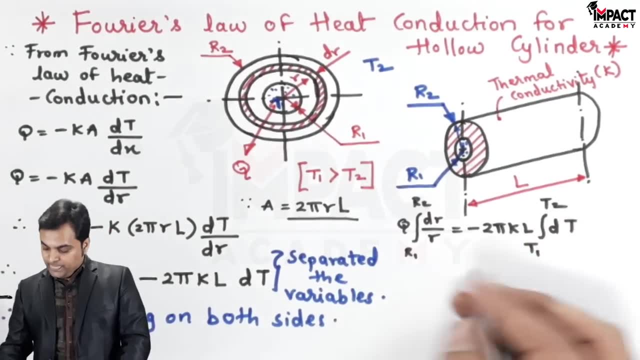 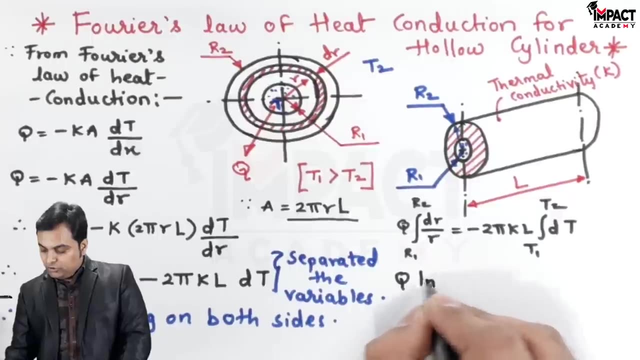 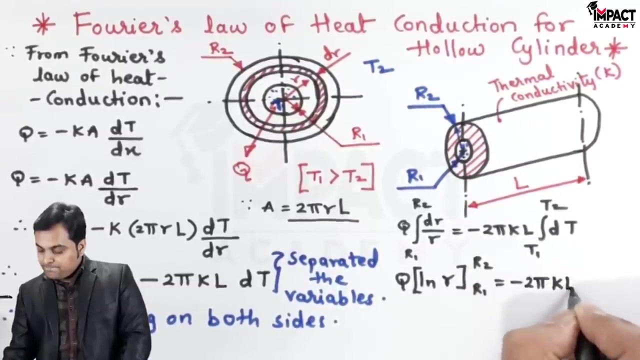 from t1 to t2, because at radius r1 the temperature is equal to minus 2 pi kl system temperature is t1. similarly, at r2 it is t2. so therefore, q will be integration of one upon r, ie ln of r and integration of dt will be t. 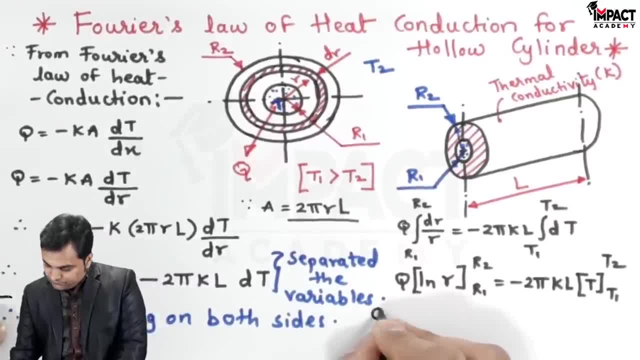 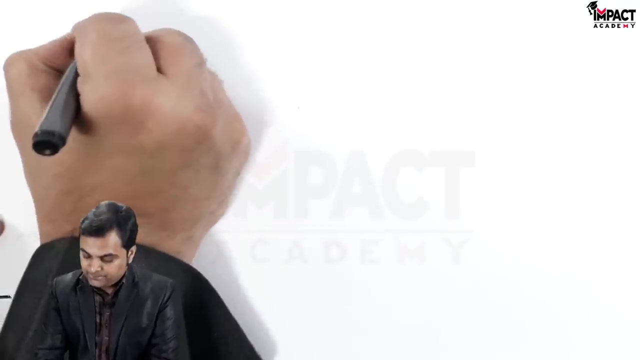 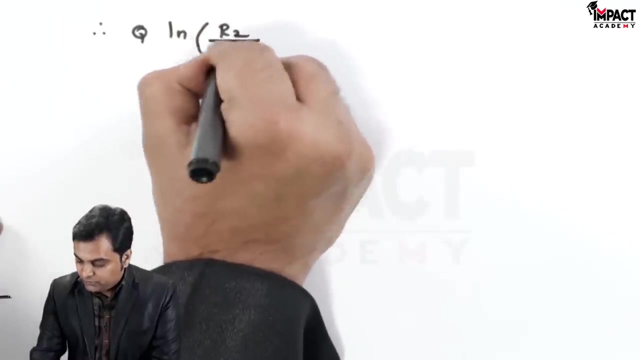 then putting the limits over here. so q would be ln r2 minus ln of r1, minus 2 pi KL t2 minus t1. then this would be written in this way: like Q is into ln of r2 upon r1, that is equal to next. 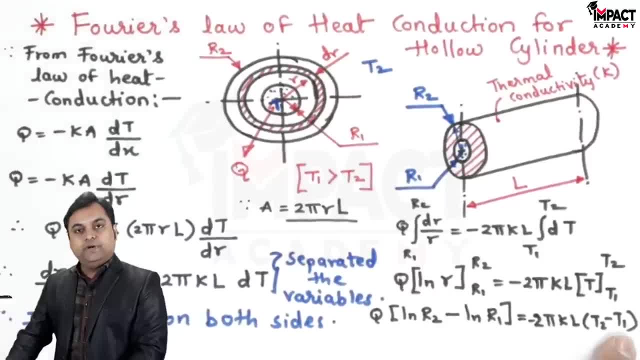 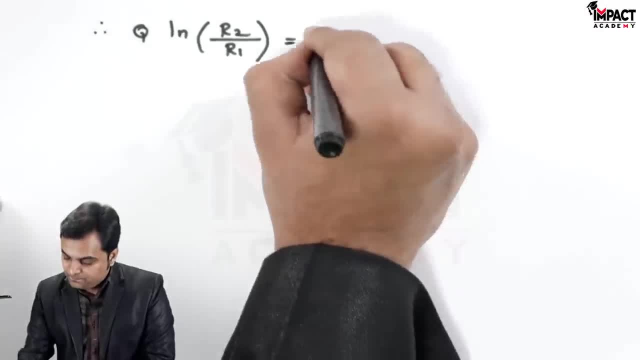 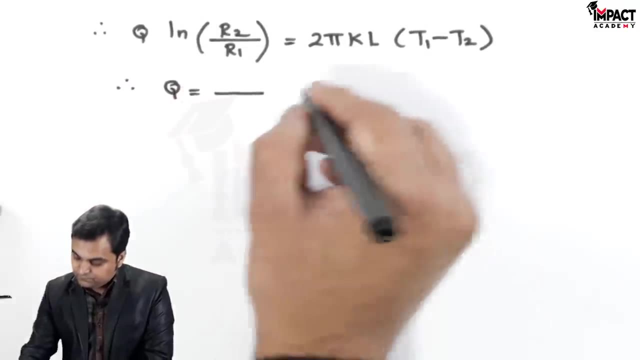 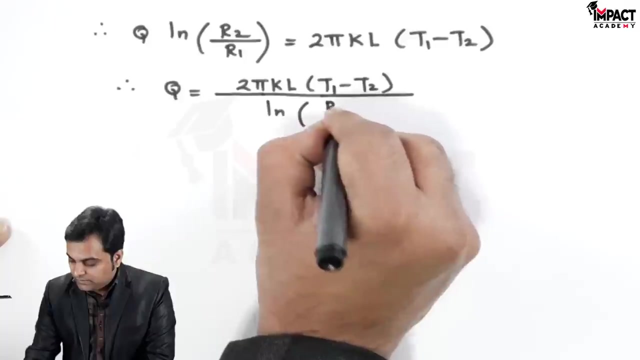 here we have minus 2 pi KL. t2 minus t1. when I put this negative sign inside the bracket would become t1 minus t2. Q would be kept on one side ln of r2 by r1 into the denominator in the numerator. I'll keep the temperature difference. 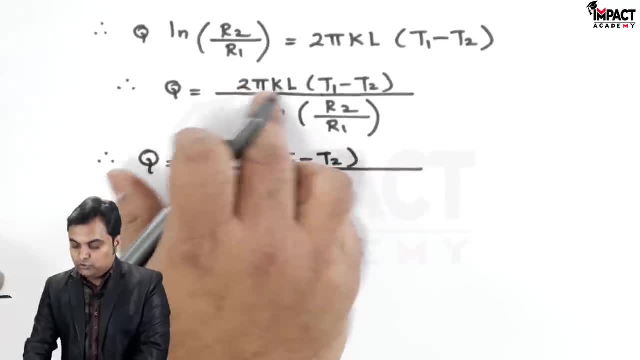 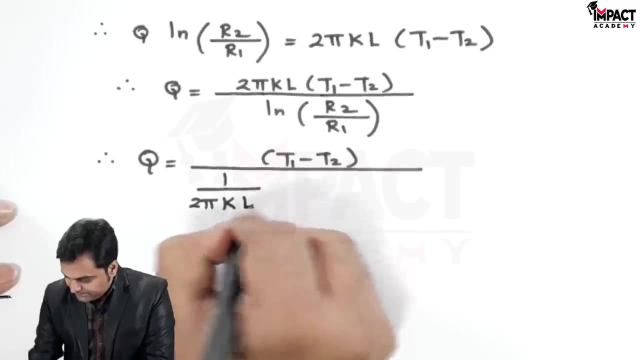 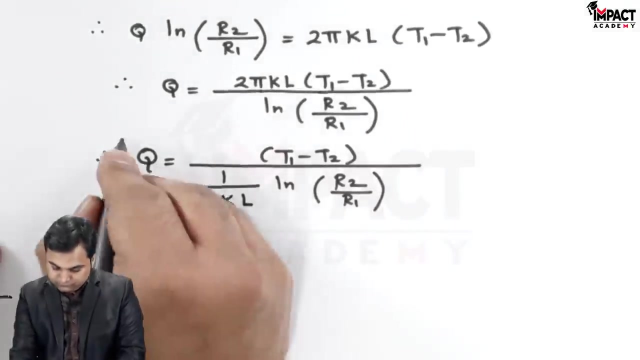 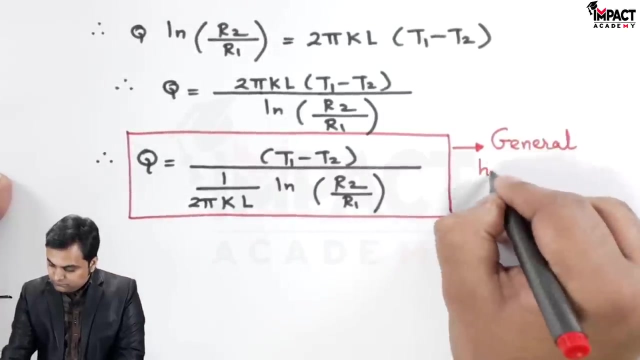 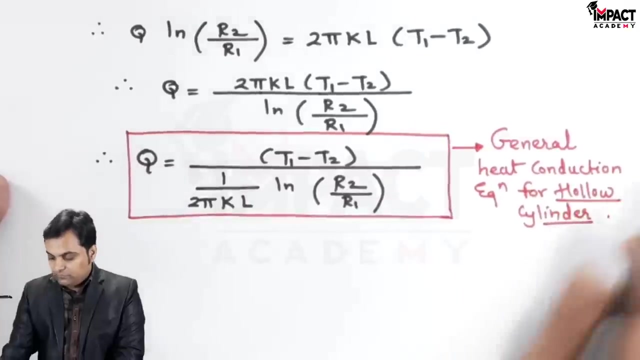 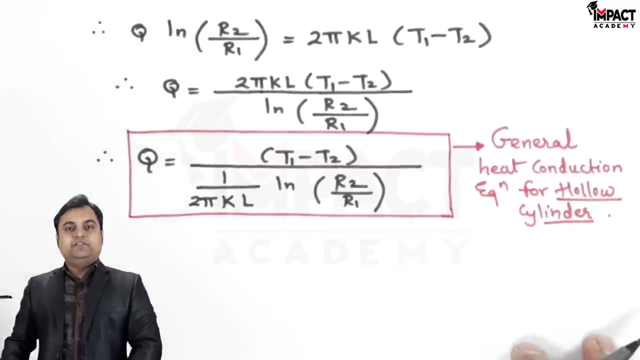 then this 2 pi KL will go into the denominator and become 1 upon 2 pi KL ln of r2 by r1. so this is the general heat conduction equation for a hollow cylinder and how to remember this formula. in the numerator there would be the temperature difference that is higher. 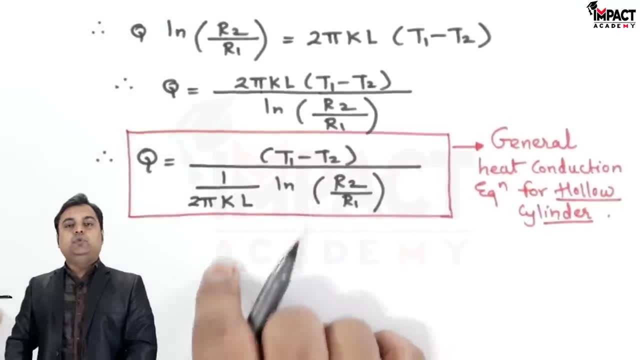 temperature minus lower temperature upon 1, upon 2 pi. KL. K is the thermal conductivity of the cylinder, L is the length of the cylinder into ln of now. don't remember the formula in the form of r2, r1, because these notations may change. so